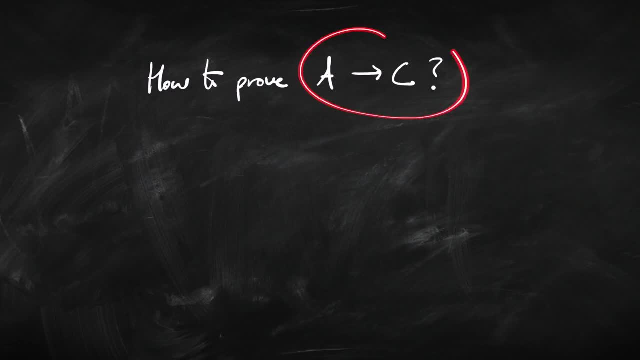 a conditional, and if, then If A, then C. Here are the steps that we're going to do to do that. First of all, we are going to assume that A is the case. Then we're going to do some reasoning, Just following the other rules, We're going to try and infer C. So we start with A and we try and get to C. 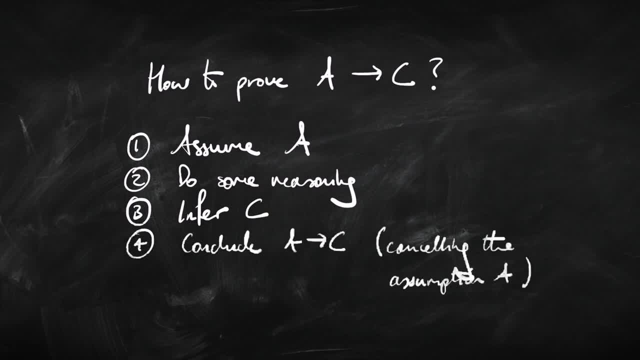 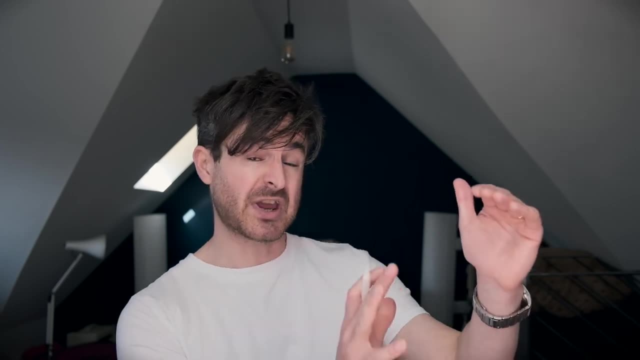 If we can do that, then we can infer or conclude the sentence that we aimed for: If A, then C. And importantly, when we infer if A, then C, we cancel out the initial assumption. we made up here that A, So let's go over that again. We're basically we're going to start assuming A. Do some reasoning Get? 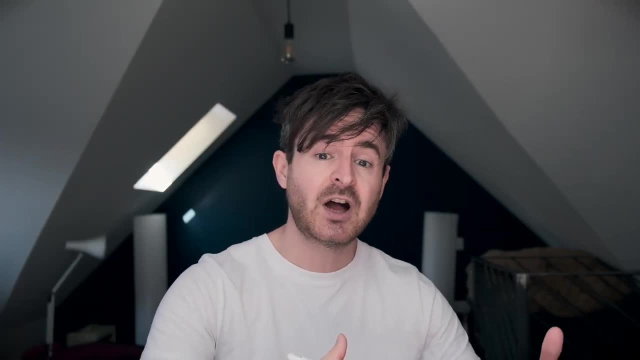 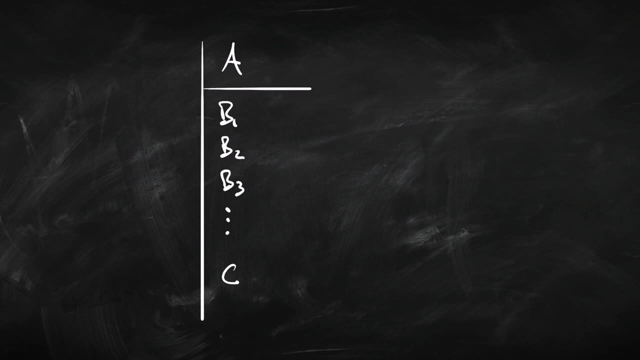 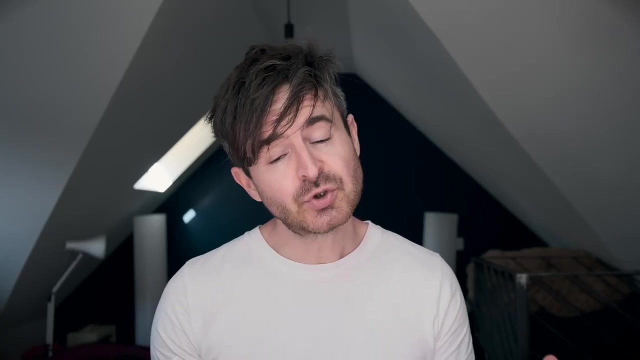 to one side, Forget about the assumption and infer: if A, then C. Let's see what that looks like in our Fitch proof notation. So previously I said we're going to have some premises up at the top, Inferences here and our conclusion down at the bottom. But this notation has a dual use. 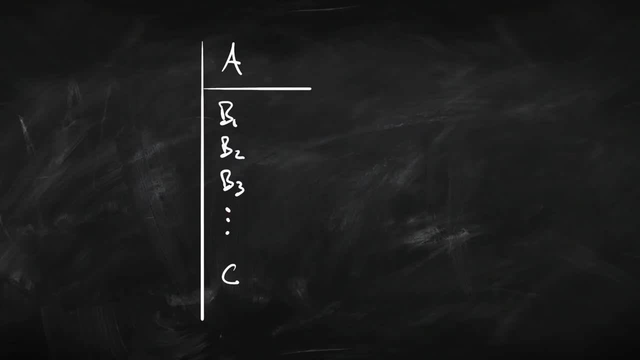 In the context of conditional proof. we're going to look at it like this: A is going to be our antecedent, We're going to assume the antecedent, We're going to do some inferences, just like before, and we're going to try and get down to C And that's going to be the consequent. Okay, so, 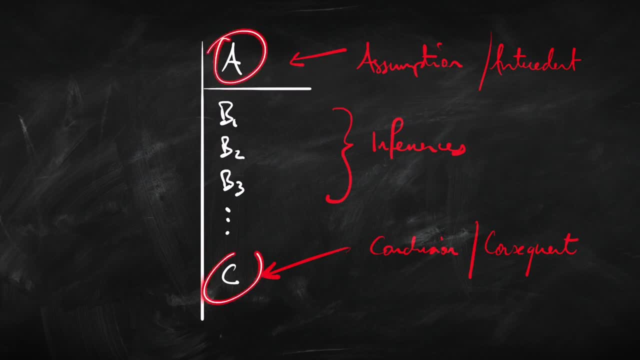 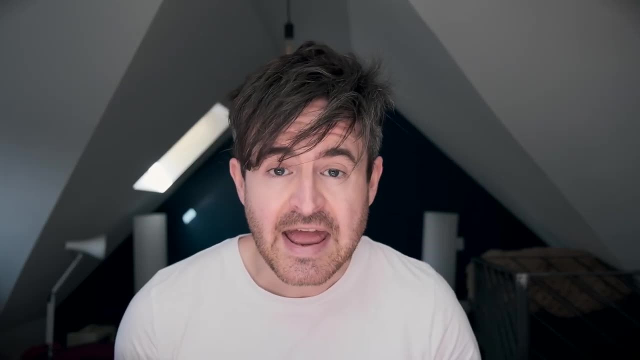 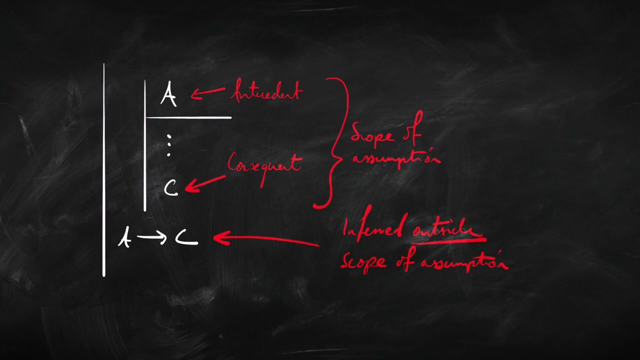 to prove an if, then If A then C, We assume the antecedent and we try and reason our way down to the consequent. So the way we would set out a proof of a conditional if A then C- is like this: We start a new assumption. So if we have a proof going on already down here we make a new assumption. 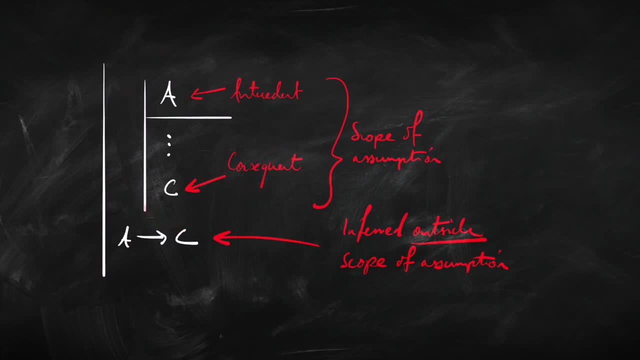 and we set it out like this: We have another vertical line marking out some new assumptions reasoning to that conclusion, the consequent of the if then. And then we conclude the conditional: if A, then C, outside the scope of that assumption. Here's the assumption, Here's the scope of the assumption, And we're trying to 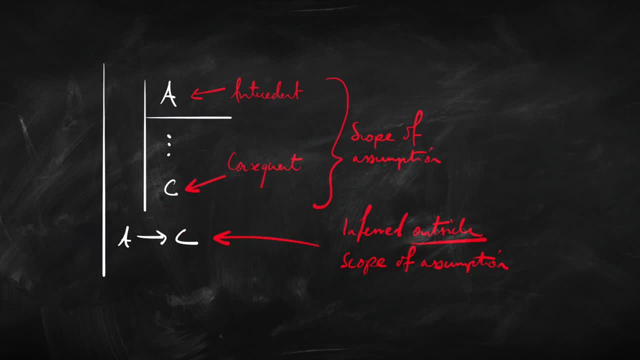 conclude: if A, then C, outside the scope of that assumption. That's the way you do conditional proof. That's the way you prove if A, then C, In Fitch style, natural deduction. So what we saw going on, there is a way that we can. 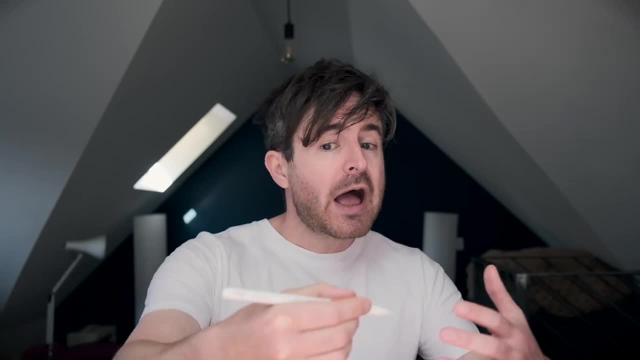 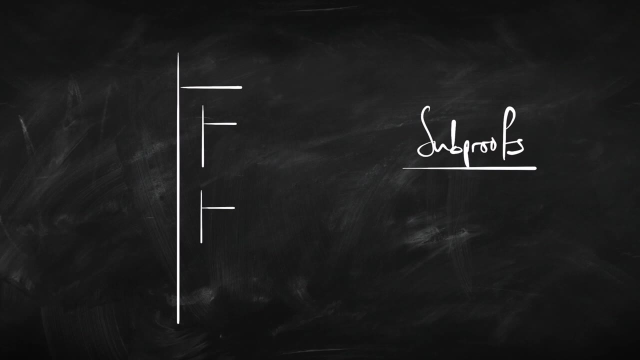 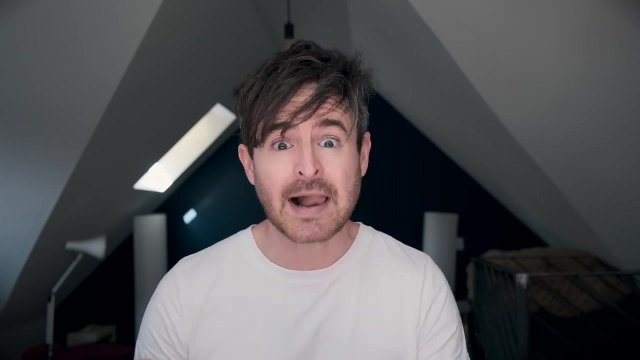 nest one proof with another. At any point within a proof, we can make some new assumptions and they can be whatever we like, And it's kind of like nesting one proof within another. Okay, so that's a very important technique in Fitch style- natural deduction. Let's just go over exactly what that. 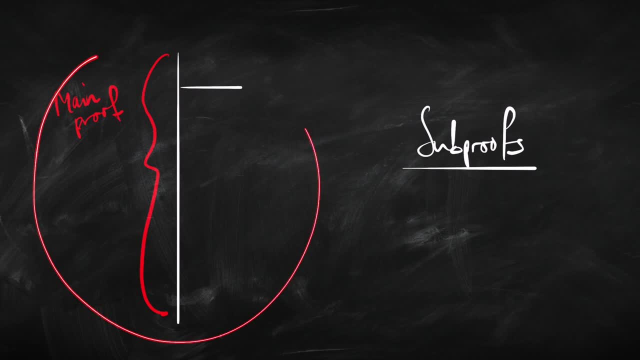 looks like We might have our main proof out here and we might have our premises- The premises of the argument we're trying to test- set out at the top here. But at any point we can introduce a sub proof by introducing some new premises, some new assumptions here, And then we do some reasoning here and then. 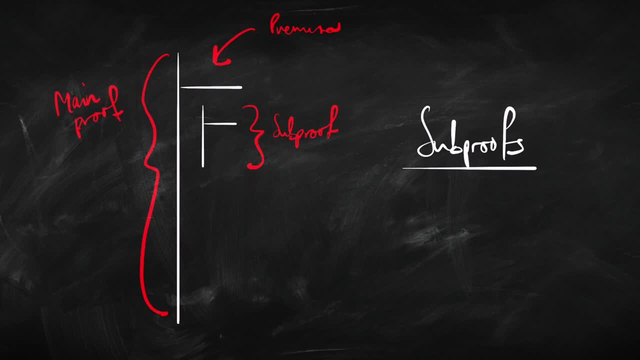 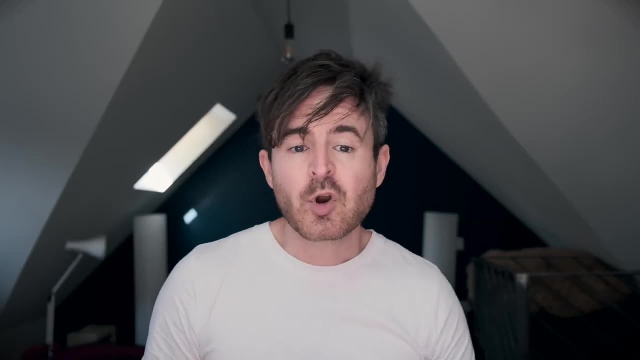 we close that sub proof and go back to our main proof And then at some point we might do another sub proof. So here would be a new assumption and here would be the reasoning. So when we talk about the scope of an assumption, here would be one assumption and here would be the scope of it. 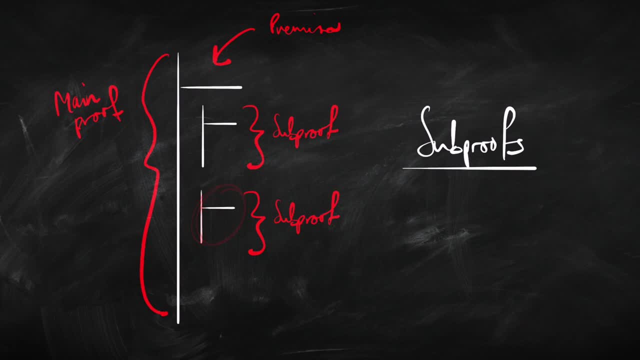 Here would be another assumption and here would be the scope of that second assumption. So all of this isn't within the scope of the first assumption. Just this is: This bit is just within the scope of the second assumption. This bit is just within the scope of those initial premises. So that's how. 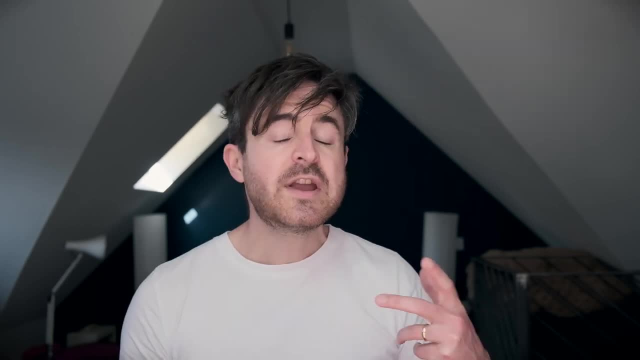 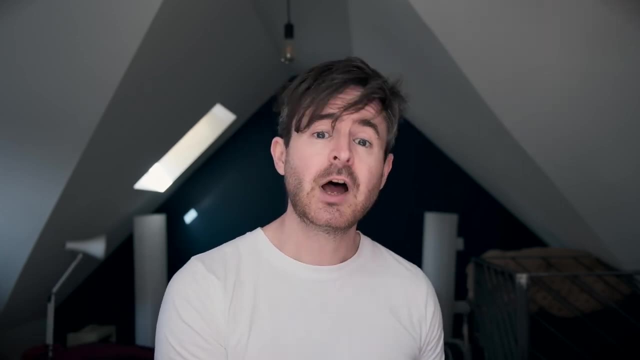 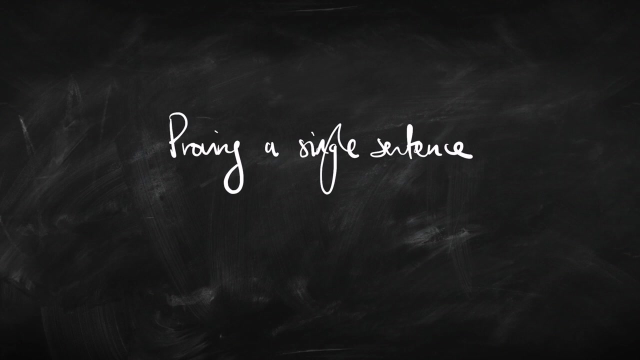 sub proofs work in Fitch style: natural deduction. We can use natural deduction to test an argument, that is, to prove a conclusion from some premises, But we can also prove individual sentences. Think about this like the case of entailment, where we have zero premises. OK, So proving a single sentence is just like proving an argument that. 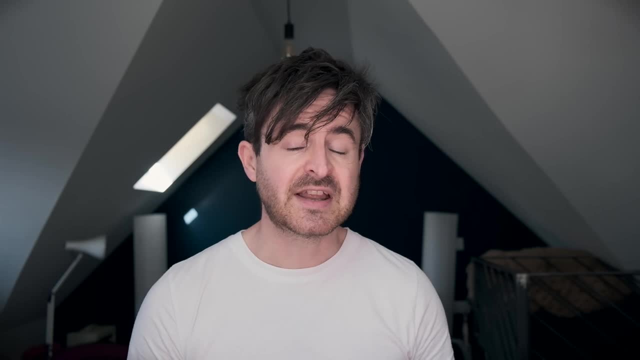 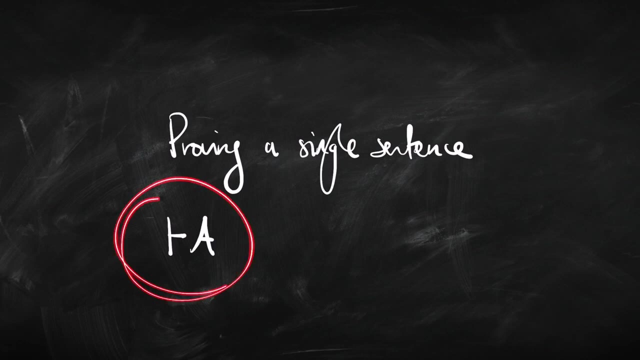 doesn't have any premises. When we're talking about a sentence being provable on its own, without any premises, we're going to write it like this: We're going to use this symbol here, which is a bit like the symbol we use for entailment, but it's just got one. 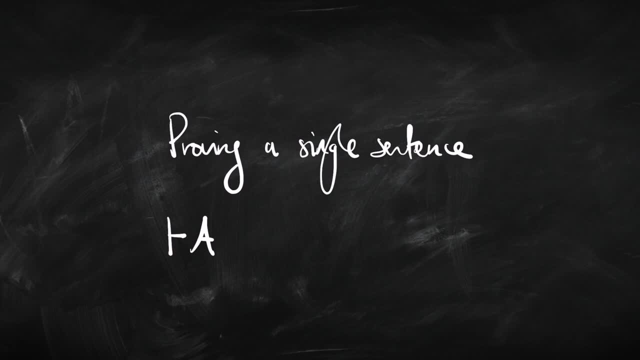 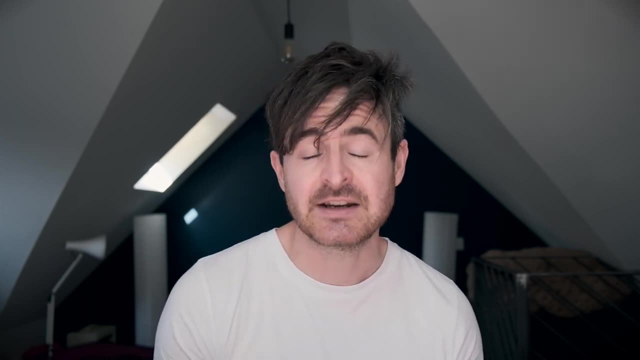 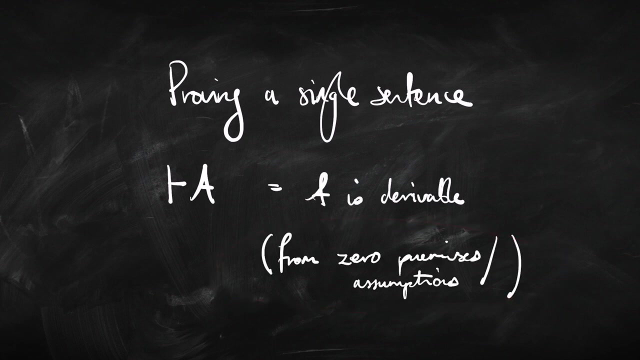 horizontal bar, So you might call this the single turn style. We're going to write this to say that A is provable or derivable from no premises, That is, from zero premises. So this means A is derivable from zero premises or zero assumptions Setting out a proof of a single sentence. A is 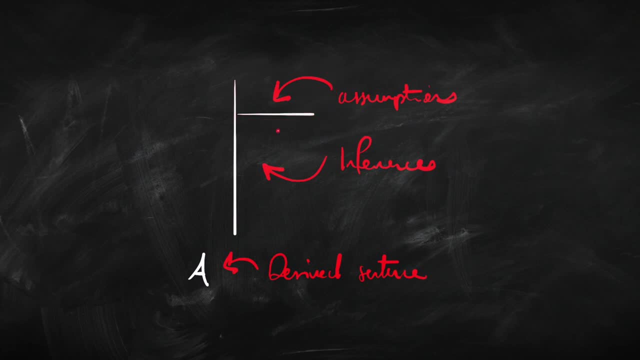 going to look like this. So at the top we have our assumptions, Underneath that line we have our inferences. And remember, this vertical line here is going to be a proof of a single sentence And A here is marking the scope of those assumptions And A here is set out to the 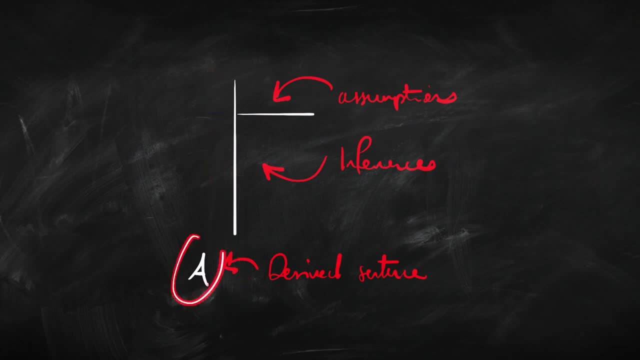 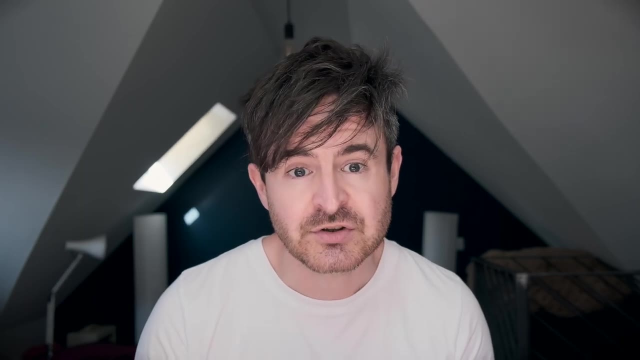 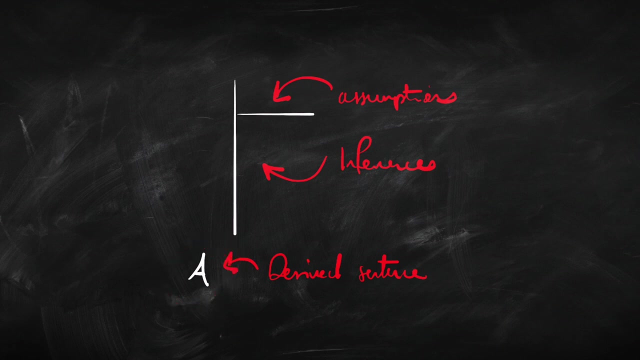 left of those. It's not within this line here. So A isn't within the scope of those initial assumptions. So we're not saying that A follows from those assumptions. We're making the assumptions so that we can do some proofs, But A stands on its own. We're not saying that A follows from. 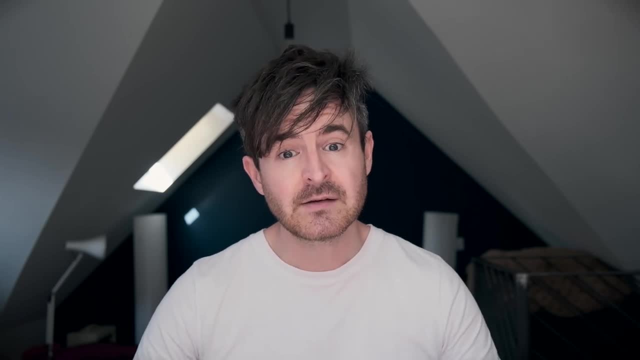 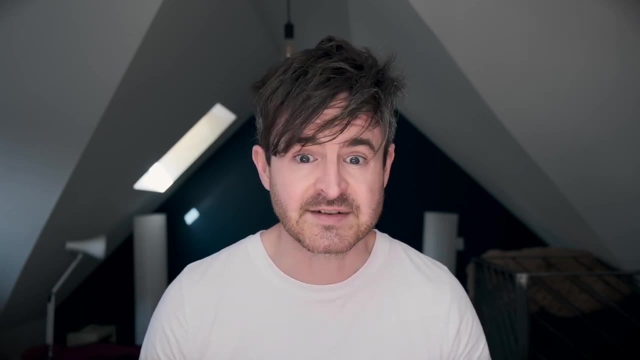 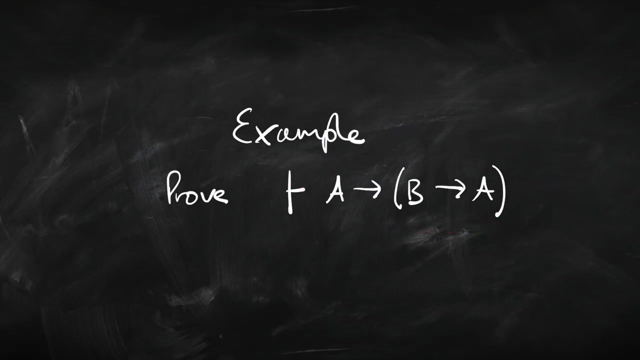 those assumptions. We are using the assumptions to derive A, But A is derivable from zero premises. It's a derivable sentence. It's a provable sentence. Let me give you an example of how that would go. Suppose we're trying to prove this sentence. It's an embedded conditional. 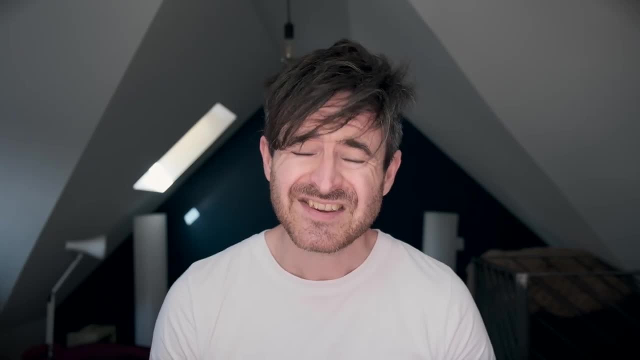 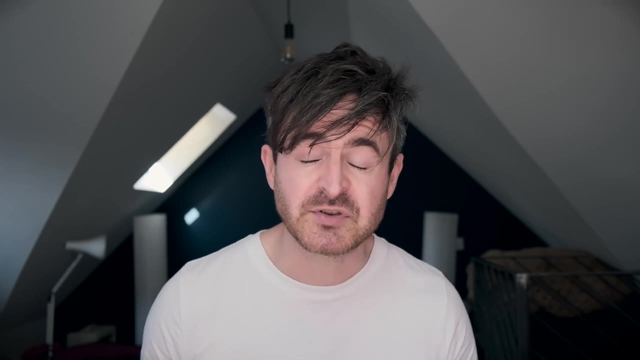 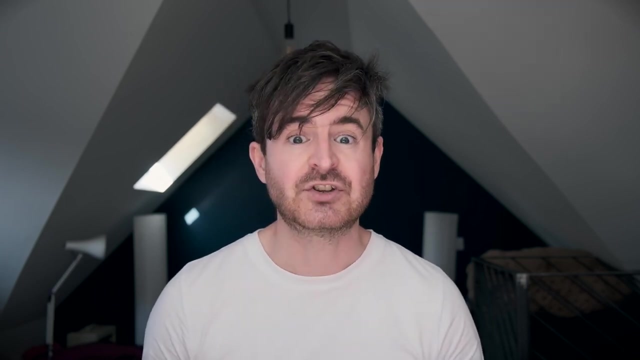 If A, then If B, then A. This is sometimes called positive paradox because some logicians think it's a bit weird, But it's a logical truth in propositional logic, in classical propositional logic, So we should be able to prove it. Let's see how we prove it in fiction. 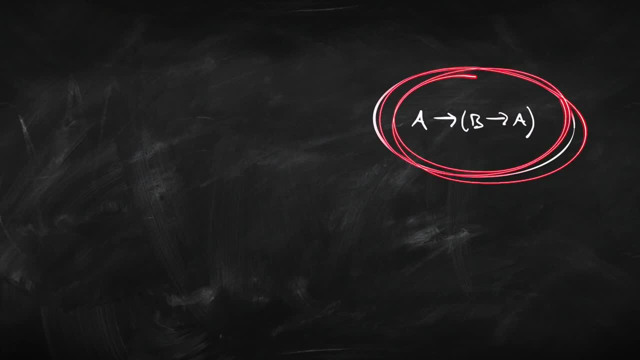 Okay, so I'm just going to write the sentence out here on the right so we remember what we're aiming for, what we're trying to prove. But this isn't part of the proof. We're going to set out the proof here in our blank paper on the left. So the first thing we're going to do is we're going to 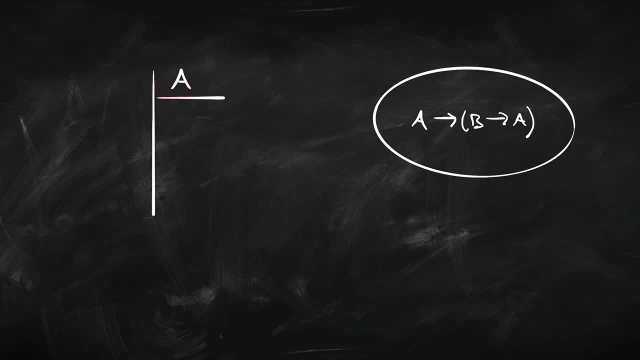 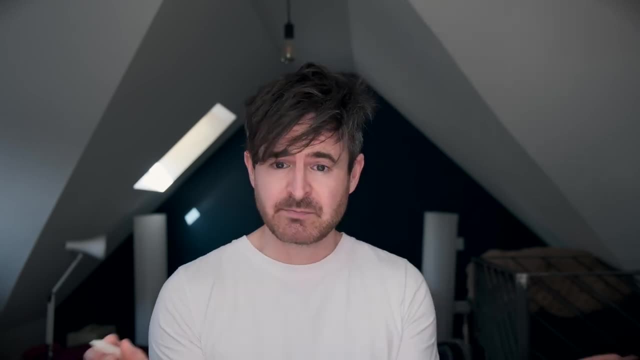 draw this shape and we're going to make our assumption A And then, immediately after that, we're going to make a second assumption B. This might seem a bit weird, but it's perfectly legit. We're basically making one assumption and then another assumption. We're. 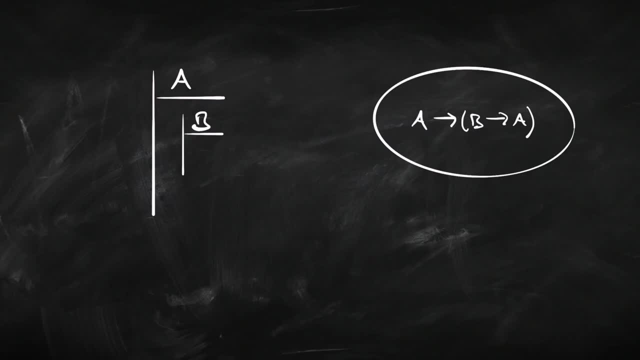 assuming that A, and then we're assuming that B. And notice, the scope of the first assumption is this bit here And the scope of the second assumption is this bit here. So within that second assumption, we've still got that first assumption that A to make use of. So, in particular, 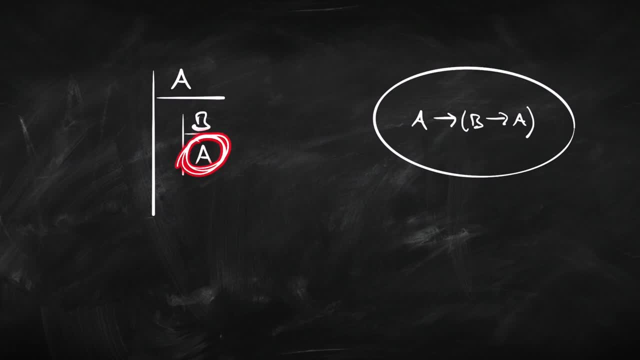 since we're assuming A here, we can have A here as well. Okay, A is still being used within this assumption here. So what we've done in this part is we have assumed B and we have derived A And using conditional proof that tells us we can infer outside the scope of this assumption.